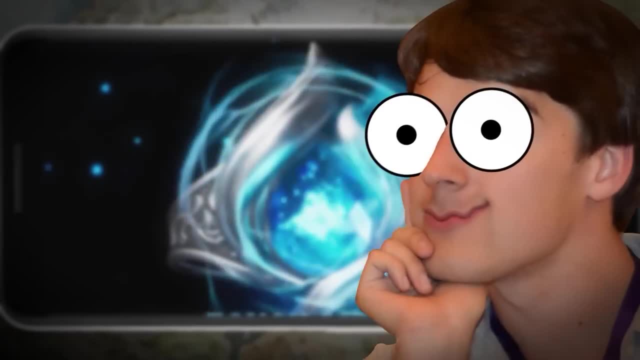 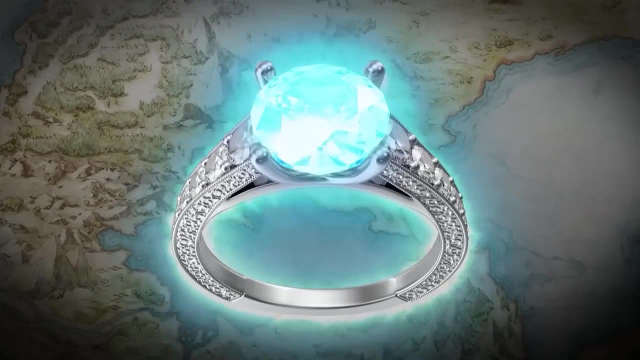 by a ring of divine power. I literally just logged on and already I'm hashtag winning, Ha. clearly this ring has got itself some excellent taste. Except there's no such thing as a free lunch Or free divine ring, I suppose. 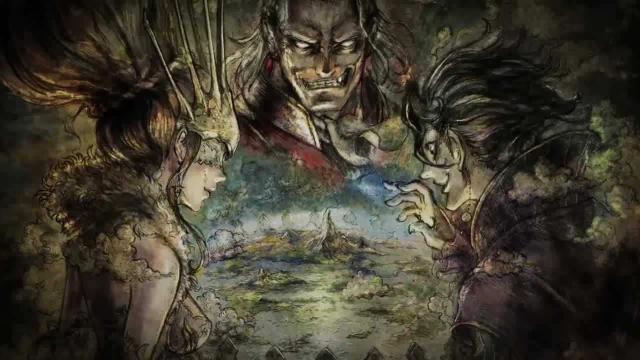 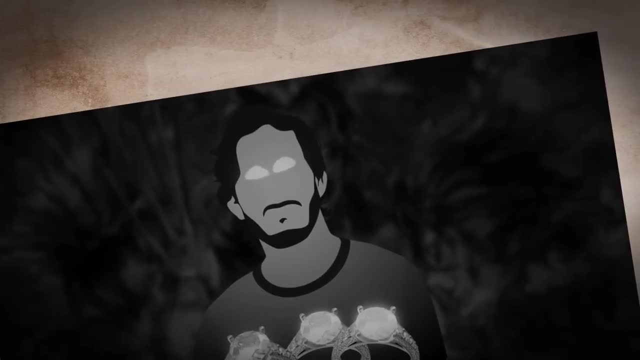 Now that you're the Chosen One, you have to take down three powerful tyrants who have their own divine rings. Only then can you collect all that jewelry, rise and become the lord of the- Well, y-y-you get the point. 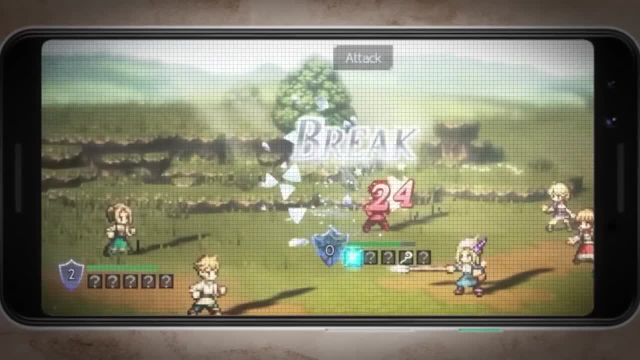 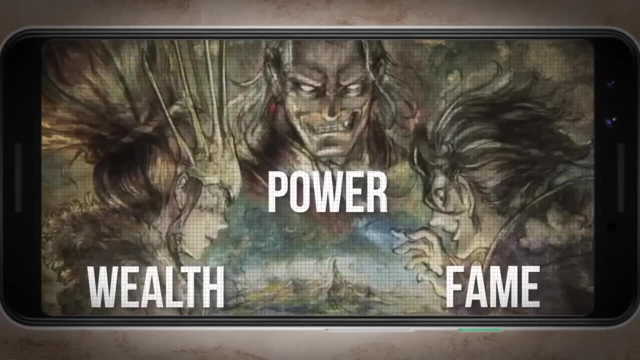 But don't worry, you're not alone. Along the way, you recruit a team of eccentric party members that'll help you when the battles get tough- And they will get tough. Each tyrant is obsessed with one key vice: Wealth, power or fame. 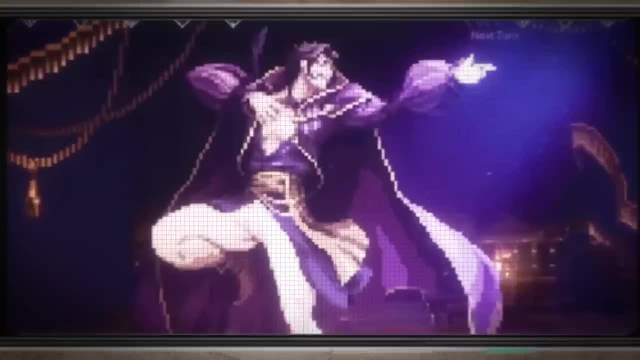 And it's up to you which order you tackle them in. Also, can I- can I just ask: Why does every bad guy in a JRPG look like the most hardcore theater kid ever? And I should know I was one of them. 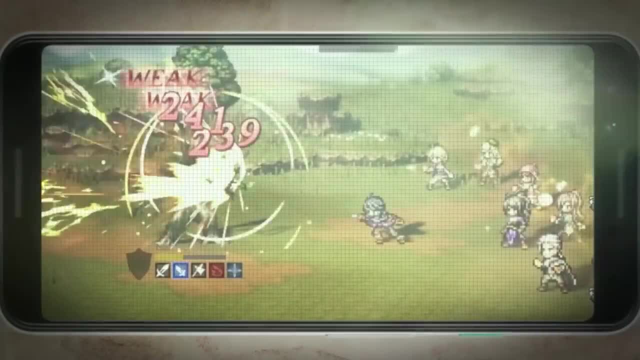 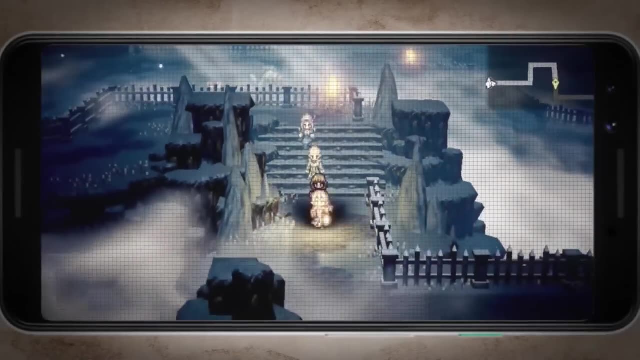 Someone slap that picture into a JRPG. The TLDR is that this game has the feel of the old-school RPGs that I loved growing up and the modern 2.5D look that makes the pixel art really pop. And, best of all, it's an honest mobile RPG. 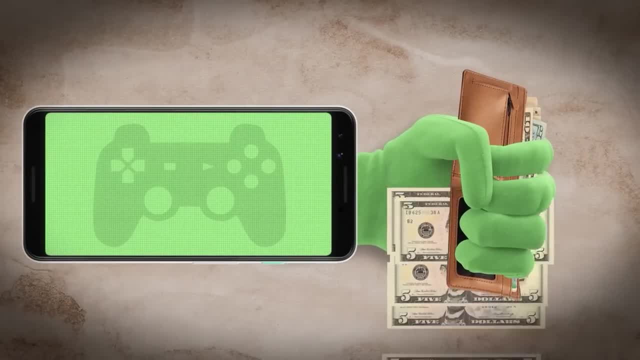 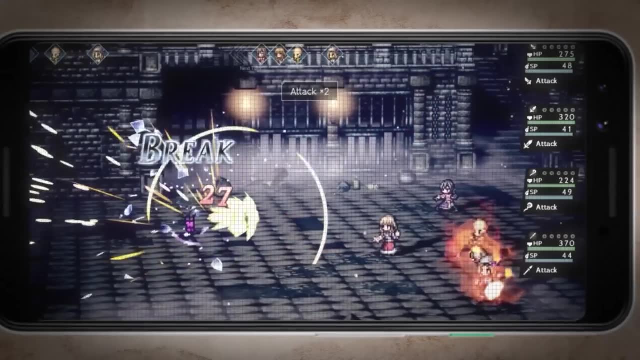 that's not designed from the outset to squeeze every dollar possible out of ya, Which, you know, when talking about mobile games, is kind of an important distinction to make. This is traditional RPGing. There's some grinding, but nothing that feels unfair. 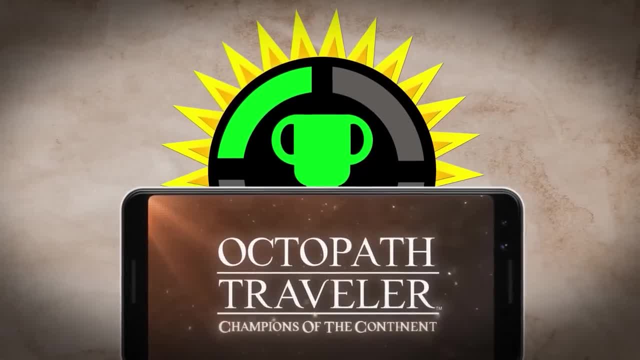 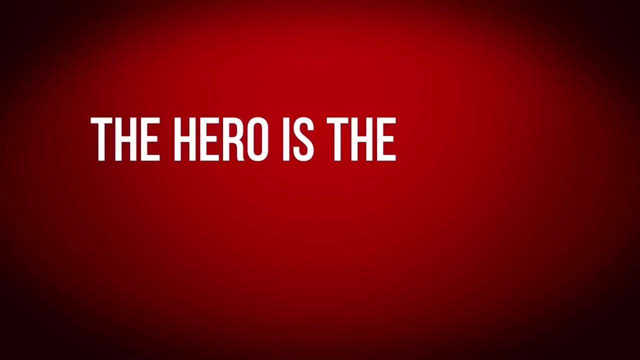 And any truly traditional RPG deserves itself a traditional game theory episode. So today I'm here to tell you that classic game theory thesis we all love so well: The hero is the villain. actually, You see, the game makes it very clear that the three tyrants we're going up against 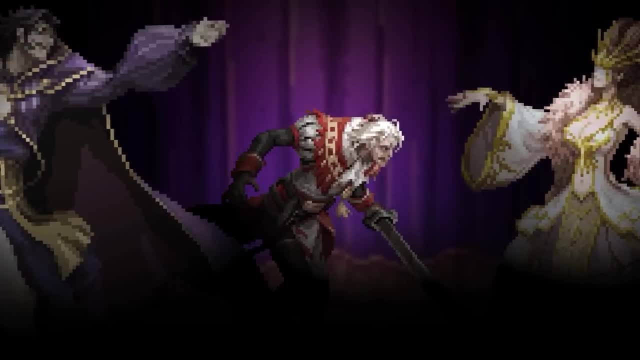 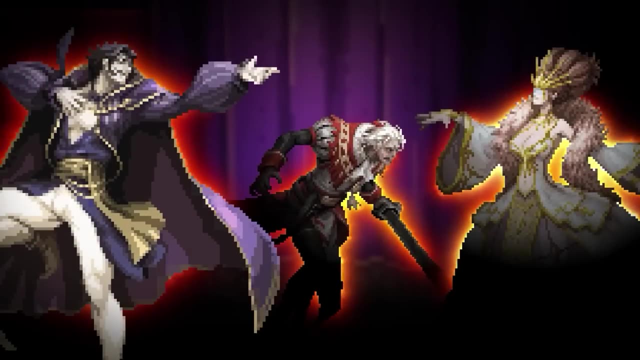 are really awful in committing all these atrocious misdeeds, But we're also explicitly told that their reigns of terror are only made possible thanks to the divine rings that they wear, which bestow upon them the power of the gods. Now remind me who else has a ring like this. 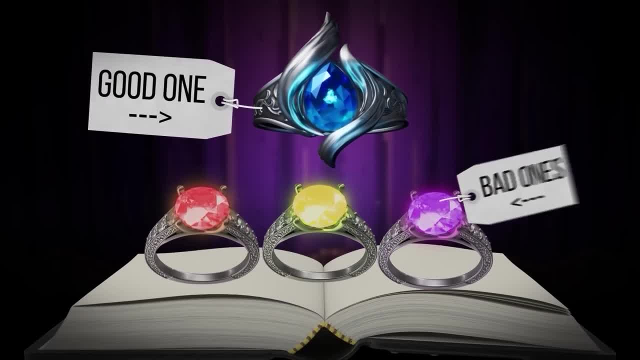 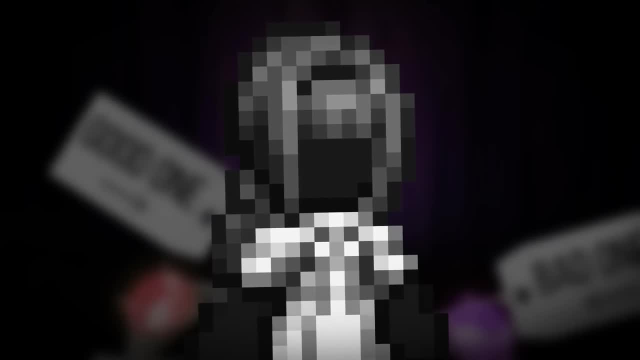 Oh yeah, it's us. A narrative storytelling one ring, just being arbitrarily different and good from all the other ones just doesn't make a whole lot of sense. And taking a look at our actions throughout the start of this game, I'm not convinced that we're all that different from the so-called villains that we're tasked with taking out. 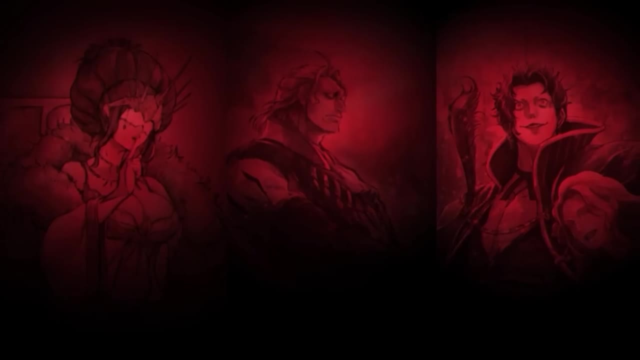 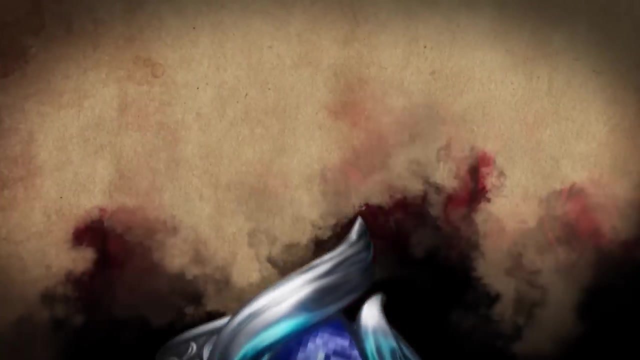 In fact, I think it's pretty darn clear: If these three were so easily corrupted by the power of the rings, then it shouldn't be hugely surprising that we also suffered the same fate. So, with all that in mind, let me take all of these branching pathways. 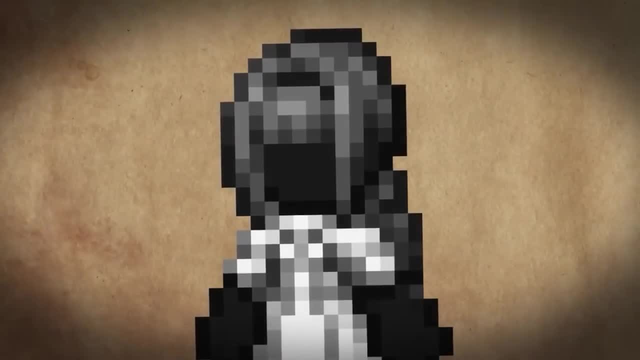 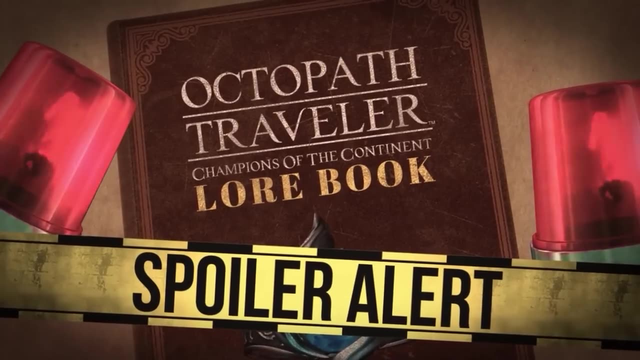 and bring them back together to show you why I suspect we are in fact the real villain of the new Octopath Traveler. Also because we're talking about some key story elements from this new game. spoiler alert from here on out. 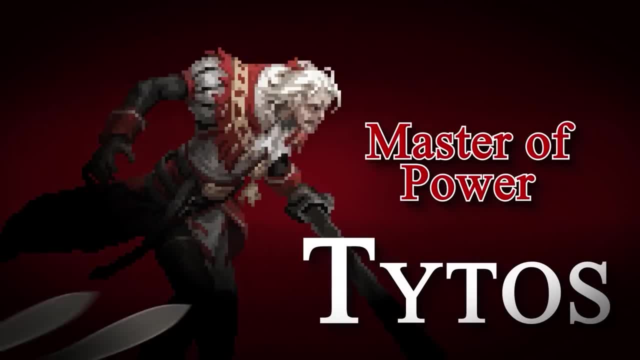 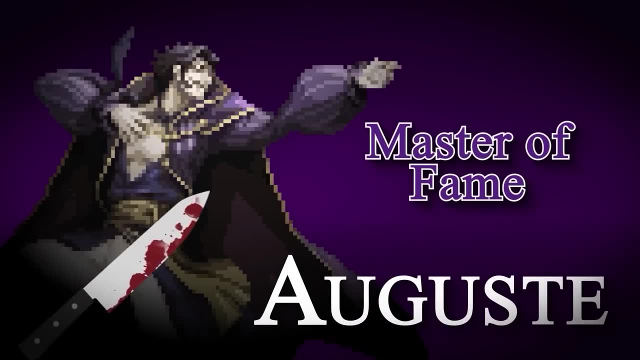 First, let's take a look at the guys that we're tasked with fighting: Titus, the master of power and the leader of a military army formed of criminals. Herminia, the master of weapons, Who runs the local mafia. And Auguste, the master of fame and murderous playwright. 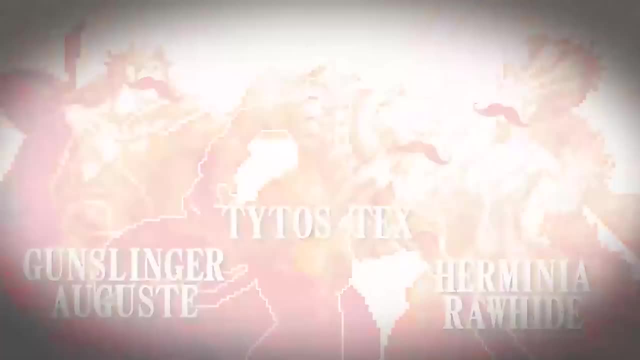 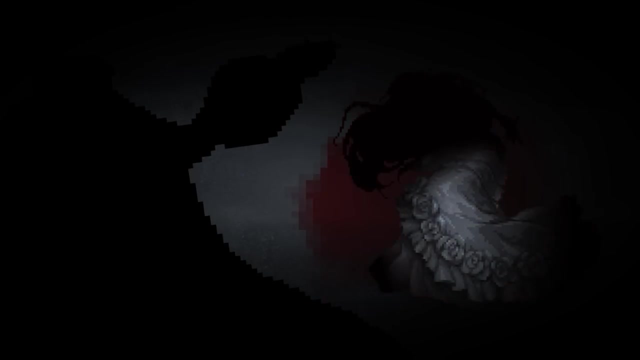 But these are far from one-note, mustache-twirling villains. Their backstories are full of tragedy and trauma. As we proceed through Auguste's story, for instance, we learn that his wife was stolen and murdered by his former boss, which thereby set Auguste on a quest for revenge. 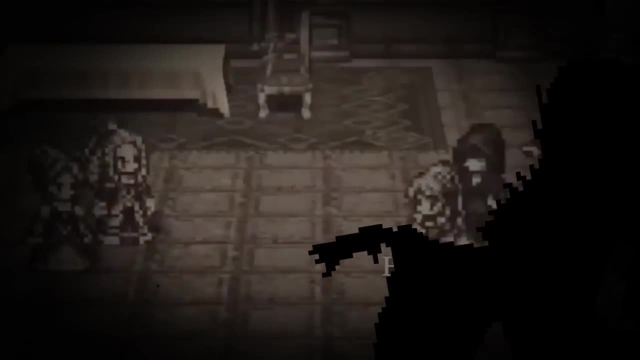 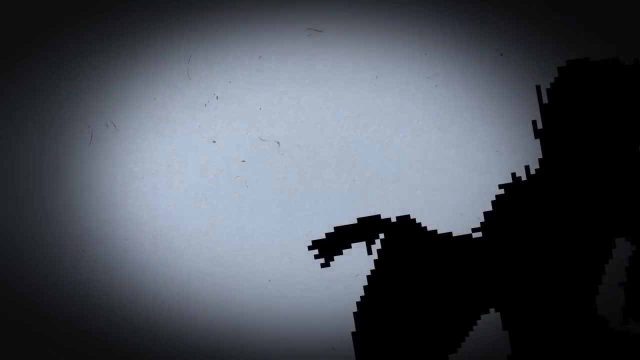 Herminia's story is even more tragic. Her sisters took her inheritance and sold her off to a distant land where she had to sell her body in order to survive. Eventually, she clawed her way up through the ranks of the mafia, ultimately becoming the godmother. 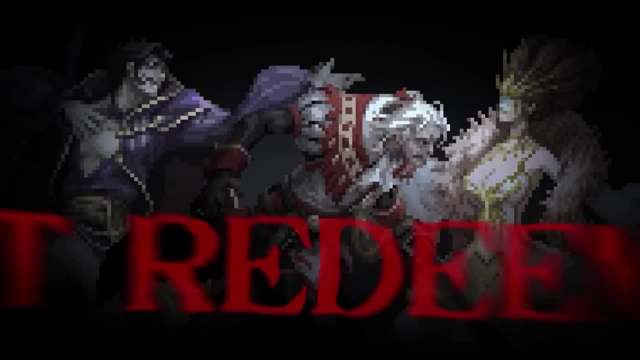 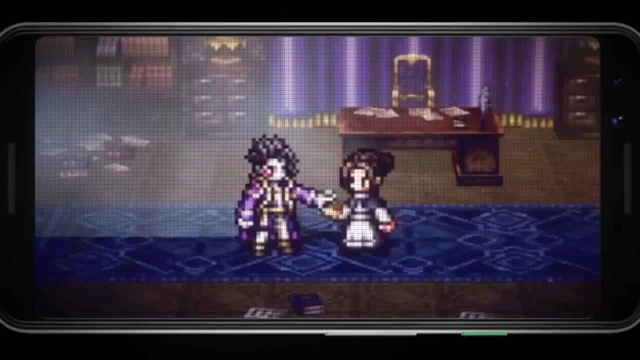 and getting revenge on her family. Now I'm not gonna sit here and tell you that these characters aren't bad guys. They are clearly killers and criminals. Their traumatic pasts don't forgive their present atrocities and they've enacted just as much, if not more, pain on others. 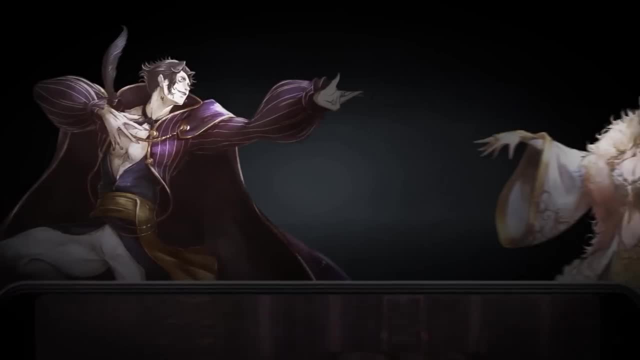 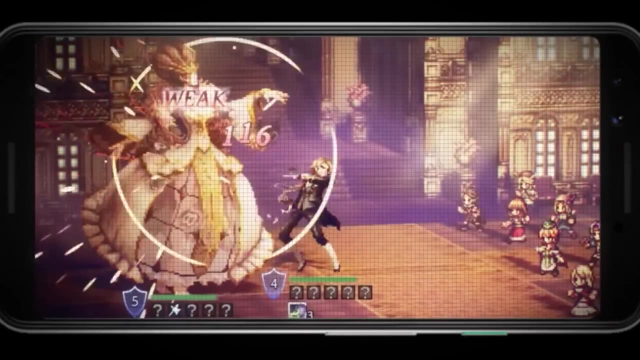 than they themselves experienced when growing up. But knowing a bit about their histories does make you think differently about how we handle the situation. For both battles we just roll up and enact our own brand of justice by wiping everyone out, And I have to ask: how is that any better than what they're doing? 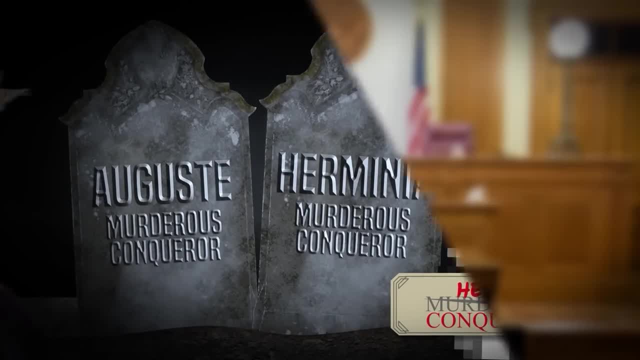 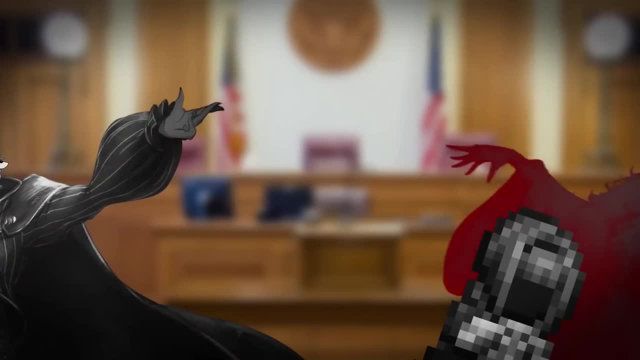 Is killing these two really the best way to stop them? At the very least, they deserve to stand trial for their crimes so the victims and the families can get closure. Instead, they get us a vigilante empowered by a divine ring striking them down. 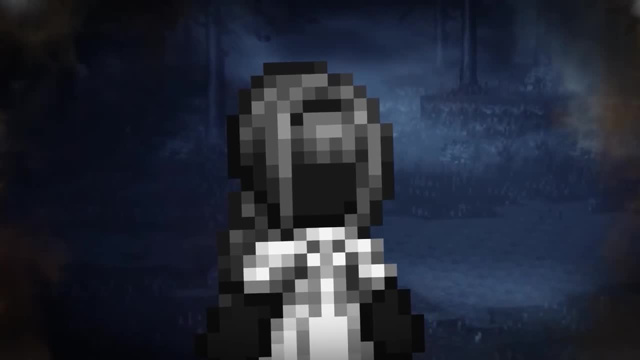 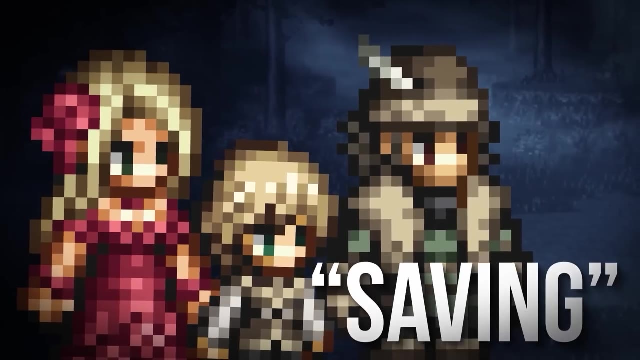 How is that any better than them? We just kill whoever we please in order to complete our mission, which is exactly what Auguste and Herminia do. It's also clear that we're not particularly worried about the people that we're- quote-unquote- saving. 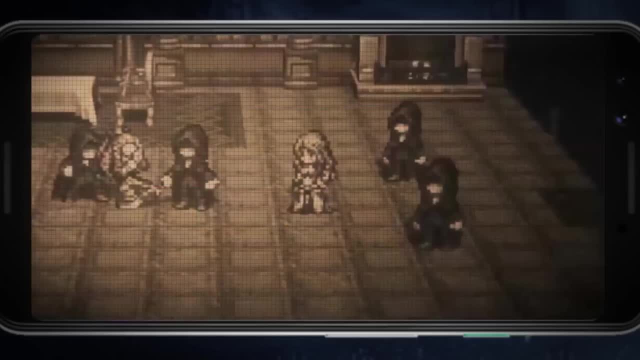 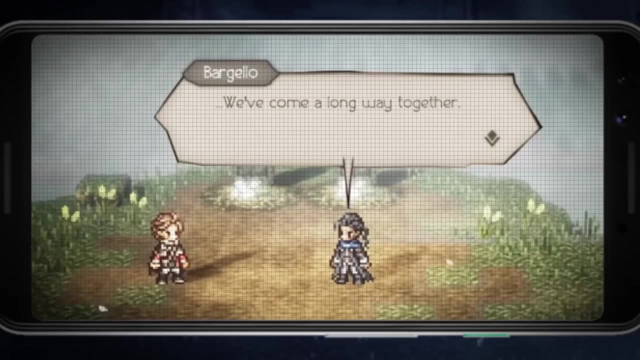 or the consequences of our actions. In the Herminia storyline, for instance, we aren't just tracking down a mafia boss. we are actively working alongside a rival mafia in an effort to put them in charge of the town. They claim to have good intentions. 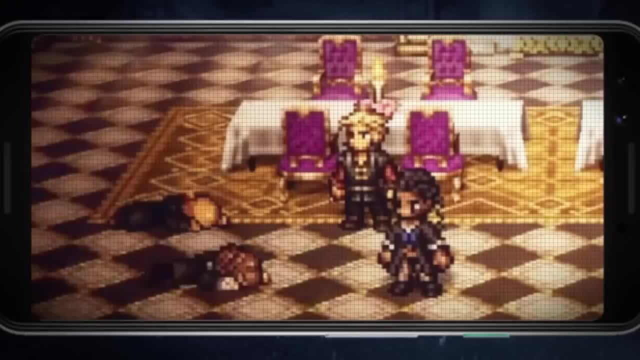 but they still call themselves the Mafia. How good can they be? And, as you'd expect, when you remove a big mafia boss from power, even if a new one takes over, there's gonna be others trying to fill the power vacuum. 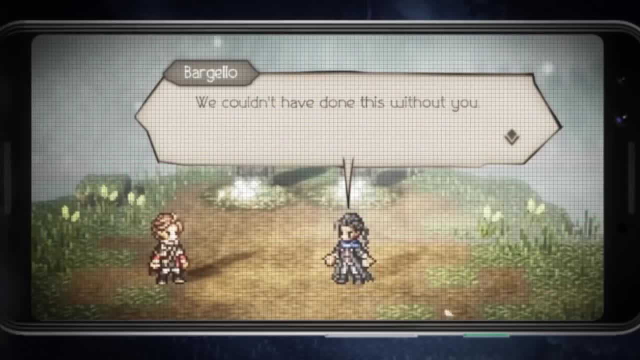 The new Don even tells us that we wouldn't have gotten this far without you. So how on earth are they gonna lead the town and survive when we move on to the next quest line? All it takes is someone bigger and badder to come along. 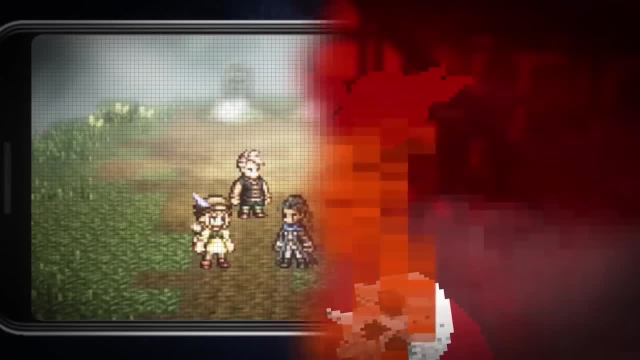 and suddenly they're gonna be done for, And we don't even have to talk in hypotheticals. Later in the game we get to come back to the town a year after we were last there and what do we see? A new big bad has entered the arena. and the government that we actively installed in the region is once again defenseless without our help. Who would've thunk it? If we truly wanted to help these poor people and their town, we'd have stuck around, Maybe helped out the new leaders to make sure everything's on track before we peaced out. 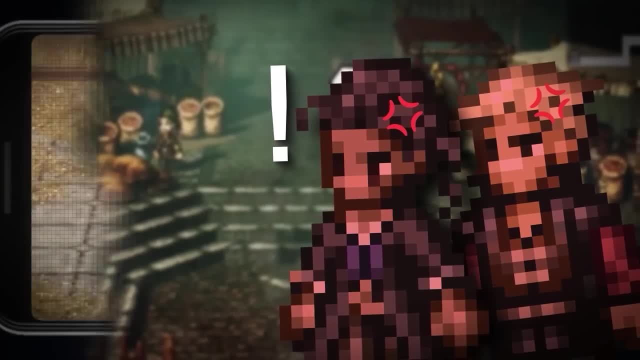 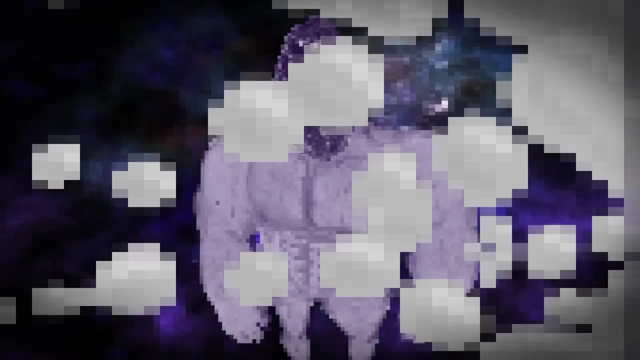 But nope, we got what we came for and we are gone. We only happen to come back because this new threat has yet another ring for us to collect. That ain't acting like a hero, friends? That is acting like a giant purple raisin man. 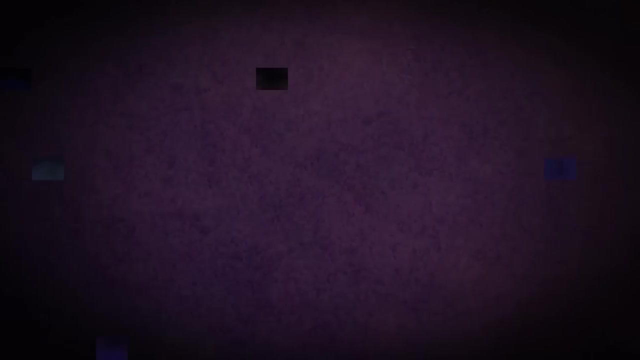 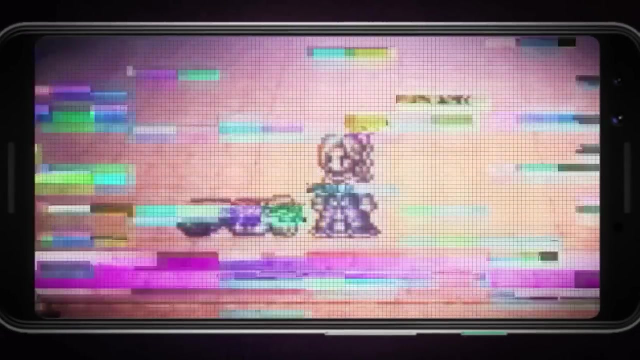 collecting rainbow gemstones for his power bracelet, Or to use this game as our example. it's literally acting no better than the three big bads. During the Master of Fame path, we meet the lead actress of a show who, we're told, 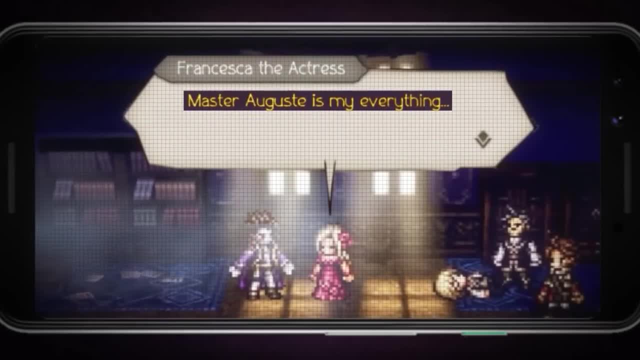 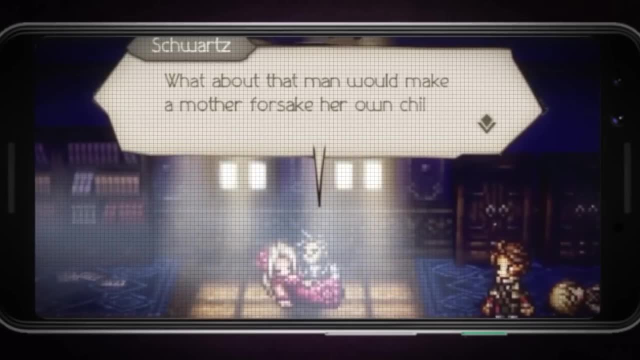 left her own son in order to follow the villain Auguste. That revelation prompts a very important question from one of our companions named Schwartz. He asks, quote: What about that man would make a person wanna abandon the life of their own child? That's a fair question. 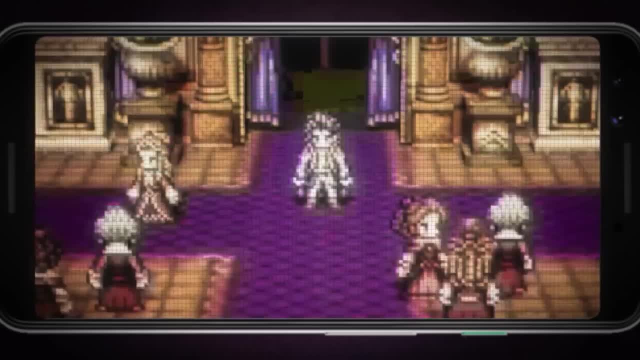 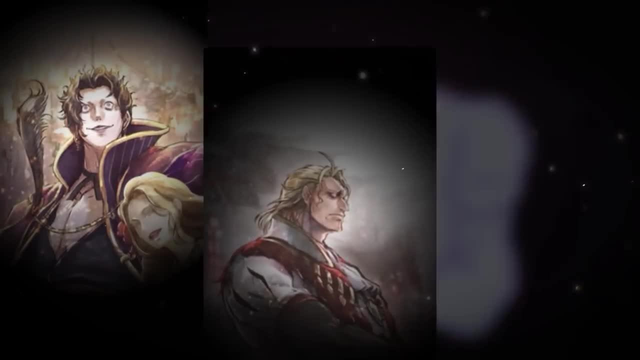 I mean, Auguste is a serial killer and yet he has legions of people loving and respecting him, following him, And this isn't the only time that we see this sort of thing happening in the game. Across all three stories, we see that the villains have accrued. 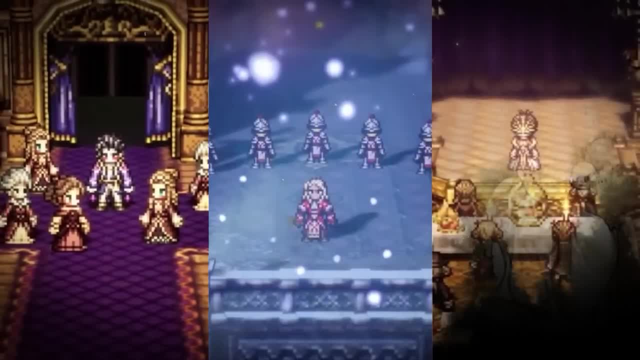 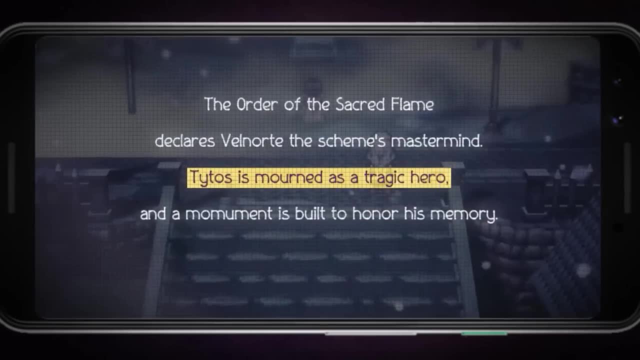 absolutely massive followings, be them fans, soldiers or people just looking for a piece of that sweet, sweet gold In the Master of Power path when we defeat the villain Titus. he is remembered by the people as a hero. Are they just that important? 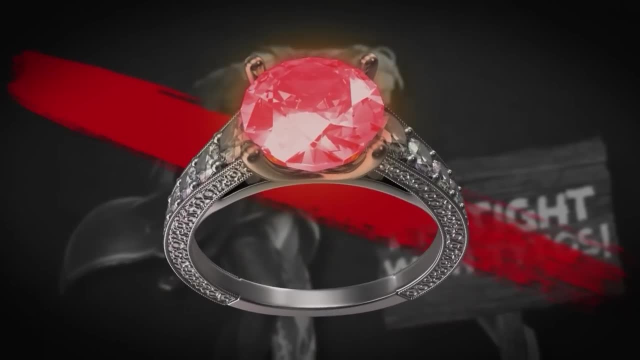 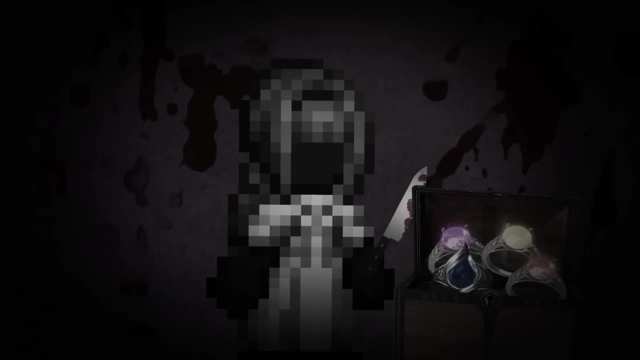 Is the propaganda just that impressive? No, I believe it has everything to do with the power that the rings give them, because when you flip the script and take a look at our player character, a random traveler from nowhere- you can see the exact. 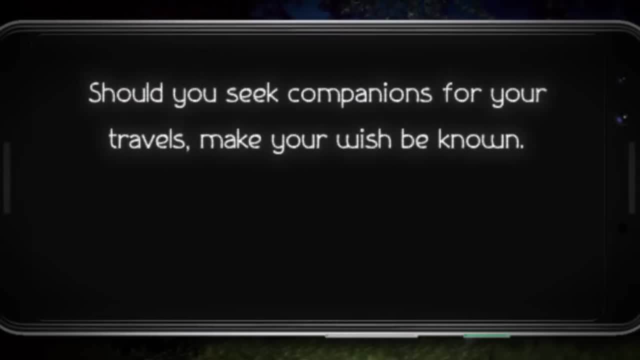 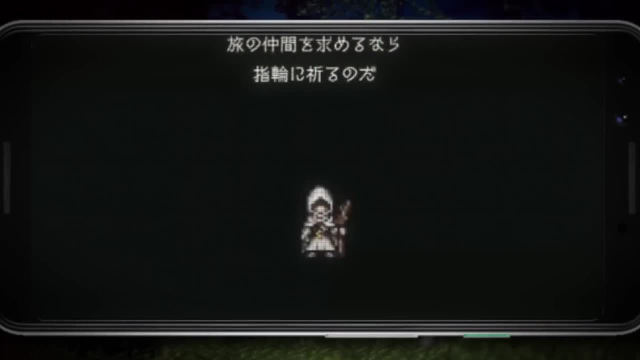 same thing starting to happen. We're told at the start of the game that, should you seek companions for your travels, make your wish be known, And you do so by tapping on your divine ring. The original Japanese is a bit more direct translating. to quote again: 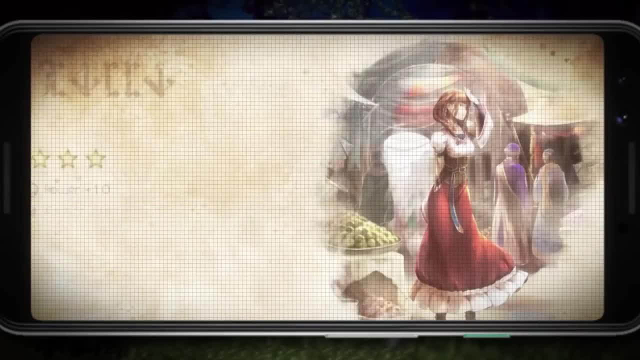 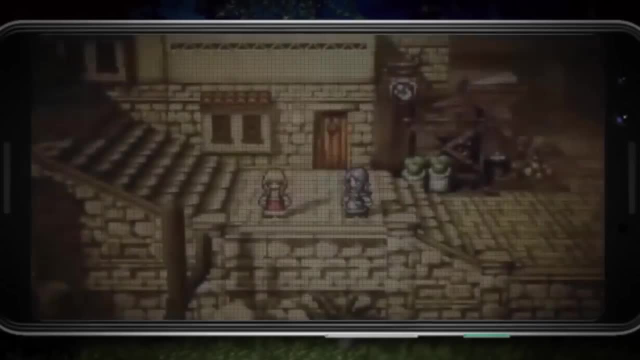 if you wish for help on your journey, then pray to the ring. When you do, you summon other travelers in order to amass a team from the 64-character roster, While these 64 characters do have backstories you have to partake in special side quests. 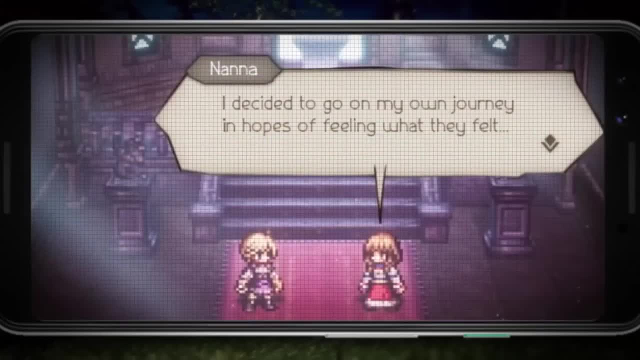 in order to actually learn them. Initially, they just show up, They give us a brief introduction of who they are, and then they're just part of your team forever, with no explanation as to why they're there. You just prayed to your magic ring. 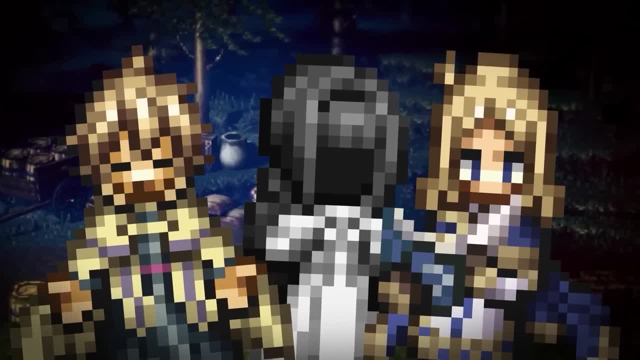 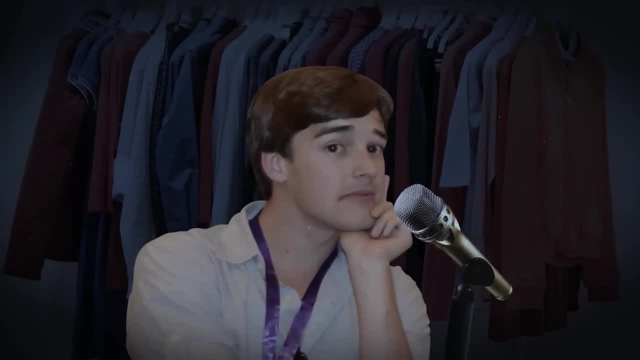 and poof, here they are ready to follow you on whatever quest, no questions asked. ready to fight any battle that you decide is just no matter how dangerous. Maybe I should get a hold of one of those magic rings. It's lonely down here in the recording closet. 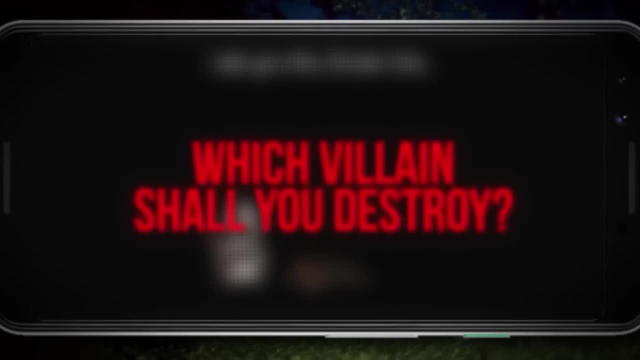 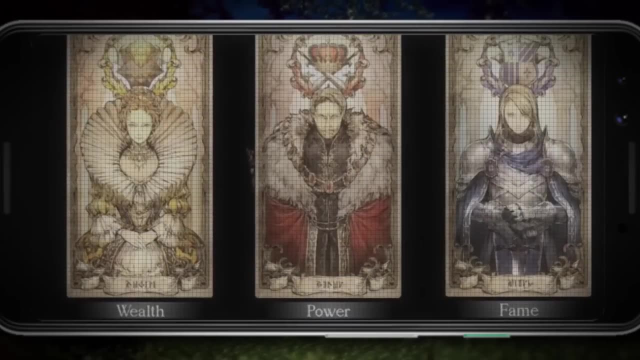 I should also point out that when you're asked to pick a story path that you want to go down, you aren't asked which villain you want to destroy. Instead, you're asked: what do you seek at journey's end, And the options are just wealth, power or fame. 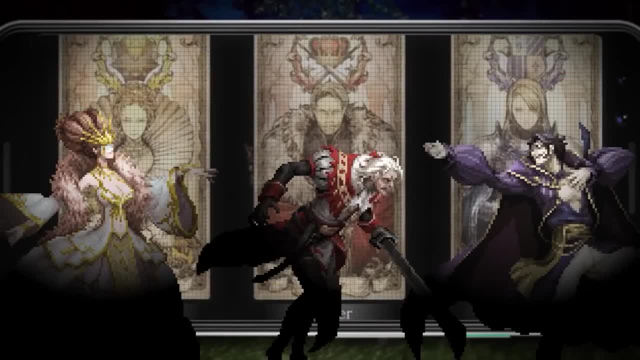 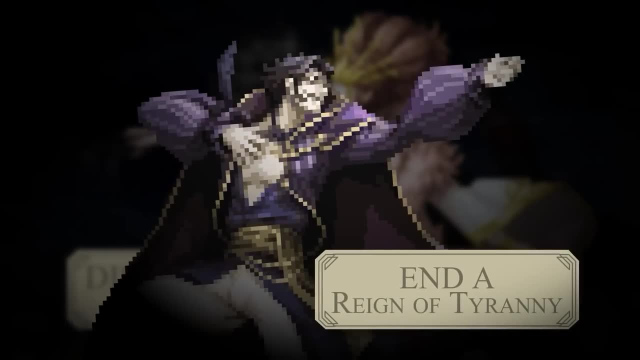 The same three things that we're accusing these villains of pursuing in their own storylines. Huh, Where are the options that say: destroy Titus or free the locals, disassemble the mafia end a reign of tyranny? Nope, none of that. 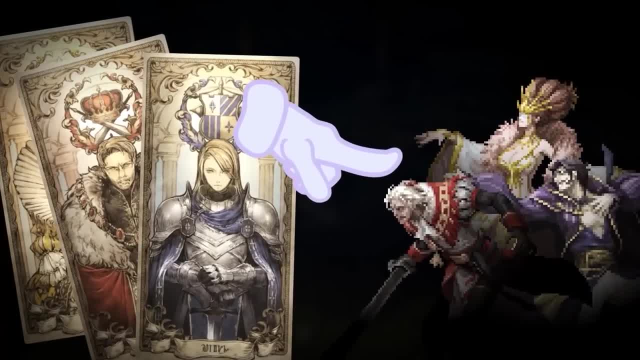 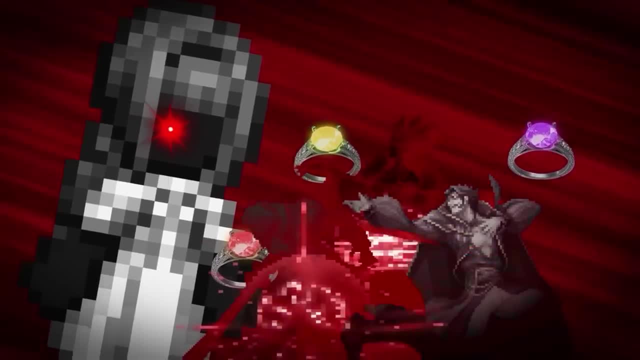 Wealth, power or fame. Make the choice. just like the villains, They all obtained magic rings and pursued one of those endeavors, And that's exactly what we're doing, too, friends. We're just going one step further in seeking all of those options. 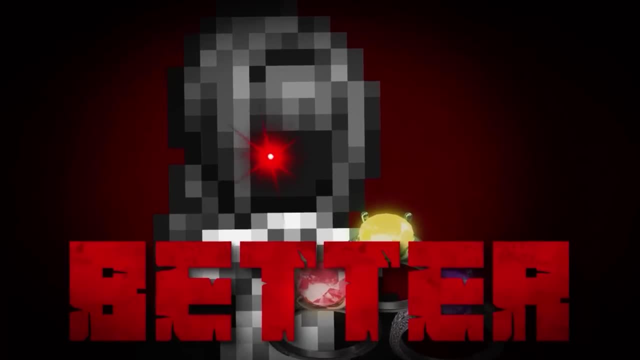 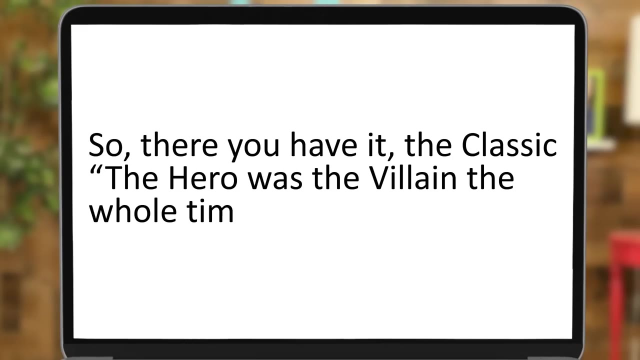 We're using the rings to do exactly what the enemies of the game did, just better: Mastering all three in order to take our place as the most famous hero in the land. So there you have it. The classic hero was the villain the whole time. 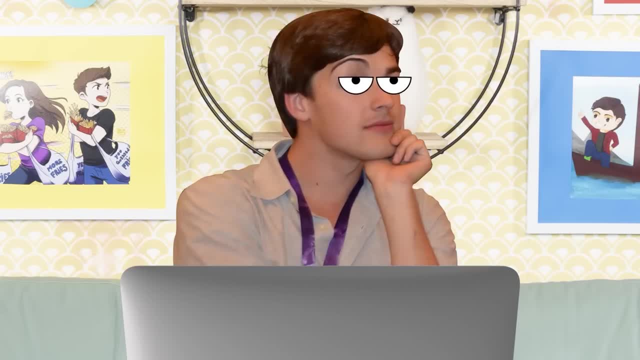 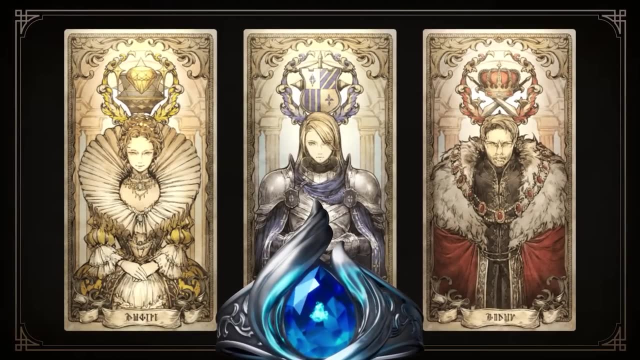 Except as I was writing that last paragraph, I realized something. We're told that these rings grant our deepest desires And our response to that is pursuing one of the three selfish goals: Wealth, fame or power. What if my heart desire was? I don't know. 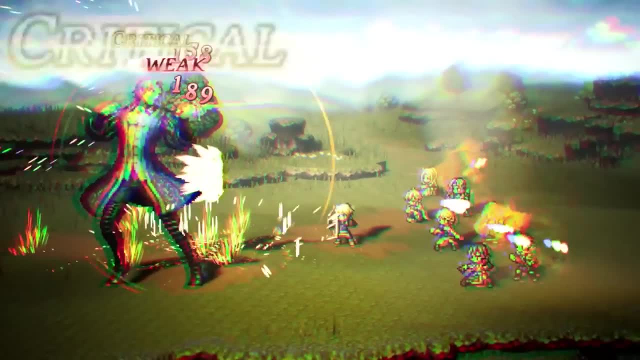 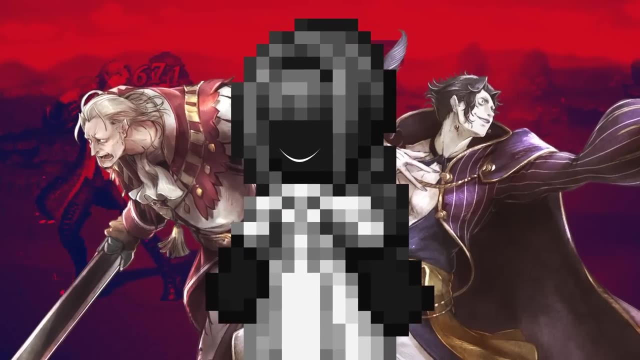 becoming a crazy cat guy or something, And we're not just pursuing those goals, we're actively plowing through others in order to get them. That means that either we ourselves are selfish and no better than the villains, or, more likely, the ring is the one controlling. 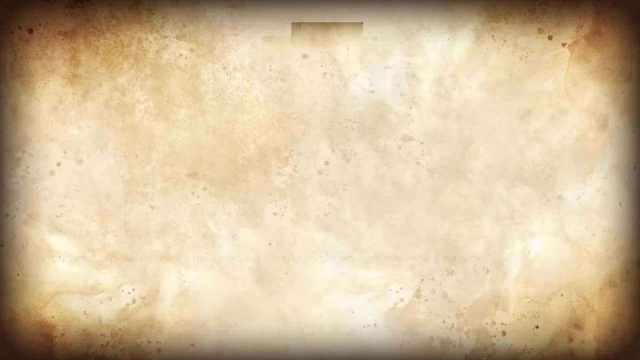 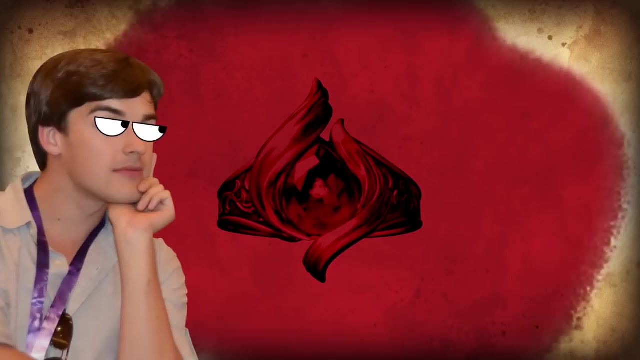 our decision in some way. Maybe the truth here is that we're not actually allowed to voice a desire all our own. Maybe we aren't the villain, the ring is. This whole thing feels like a trap that's set by the ring, Like we're being pushed into a desire or path. 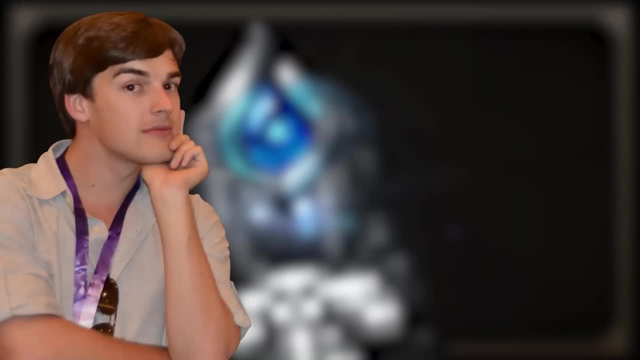 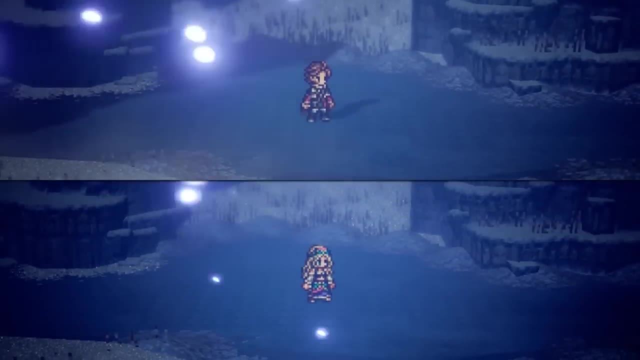 that my character may not actually want to take. I wanted to go a little bit deeper into this, so I actually restarted my game just so I could go back through the intro cutscene, And when I did, something strange happened: I was now looking at a totally different character. 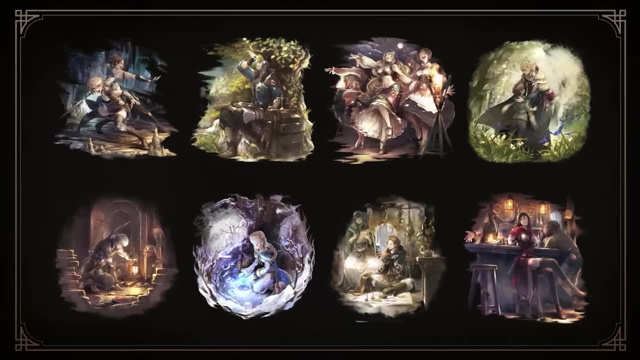 I looked it up and apparently this is an intended mechanic: Everyone that plays gets a different starting character, which I suppose allows for unique and interesting team building, But it also presents itself as a different character. But it also presents itself as a different character. 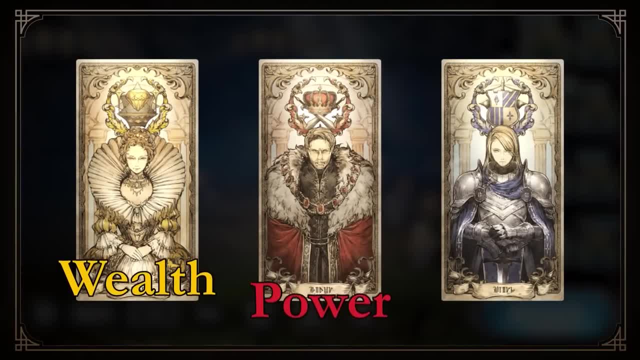 But it also presents itself as a different character. Each game gives you the same choice: Wealth, power or fame- But that can't be right. If you gathered eight random people into a room, the chances of all of them wanting the same thing, 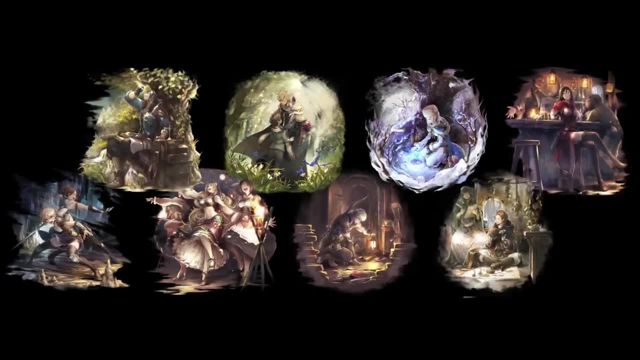 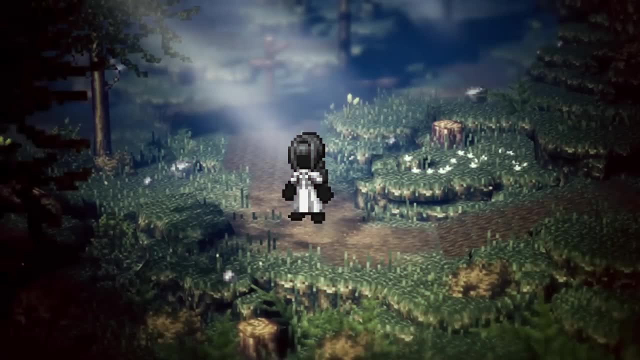 for their heart's desire are next to none. However, what's the one thing that unites all of these characters? What's the one thing that they all have in common? when you start the game, They're given a divine ring. All this time, I've been accusing the chosen one. 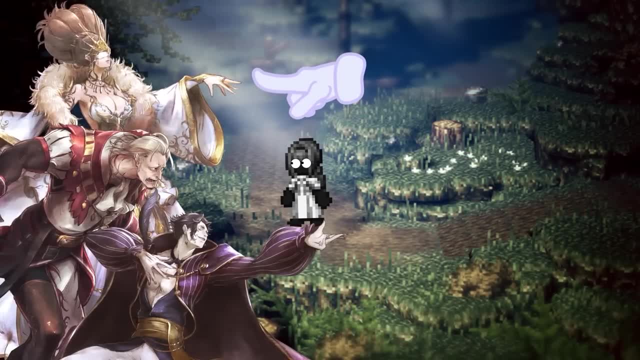 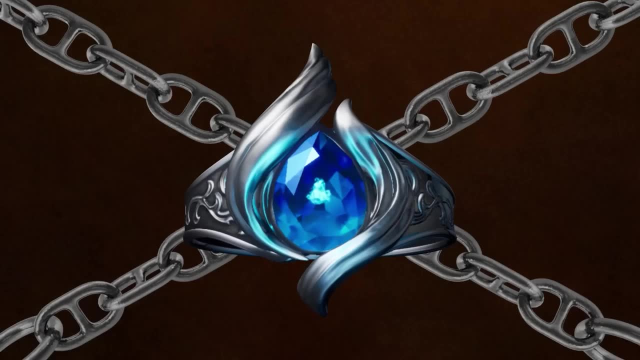 of not being a hero, that their desire is worse than that of the villains that we face throughout the initial story. But if you can literally be any character at the start of the game, well, this just proves that the ring is actually the one steamrolling our options. 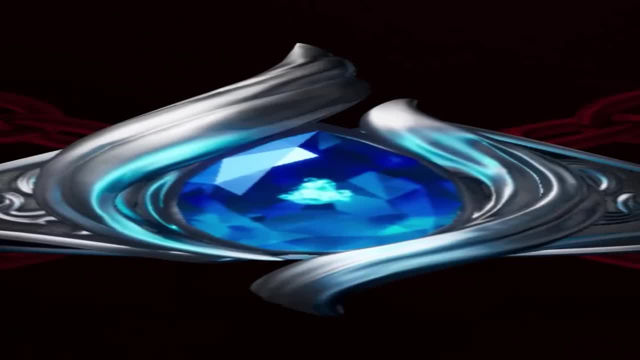 It's corrupting us from the opening seconds. Now I know this might seem like a stretch to say that the ring is somehow controlling all these people, that it's just a gameplay mechanic, but you don't have to take my word for it. 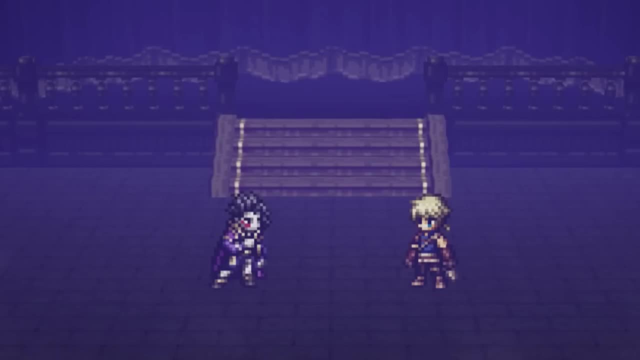 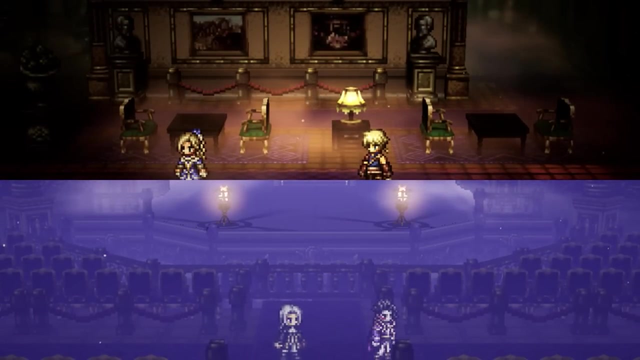 Auguste basically tells us this: after we defeat him and take the ring away from him: Finally the ring free from that abomination, I am released. Throughout his story we're told not once but twice, that Auguste has no desire for fame. 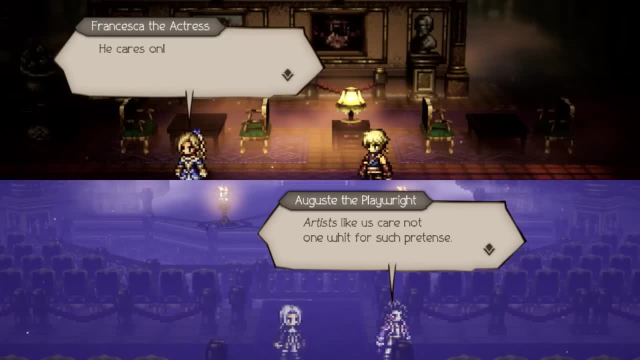 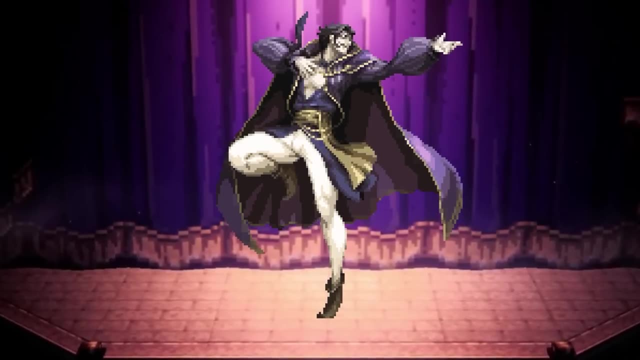 despite being the master of fame. In fact, he refers to fame as snobbery. He's an artist. He wants to create amazing plays to help reveal the desires of man through his work. He is not doing it for the fame, but the ring is the thing that's forcing him to. 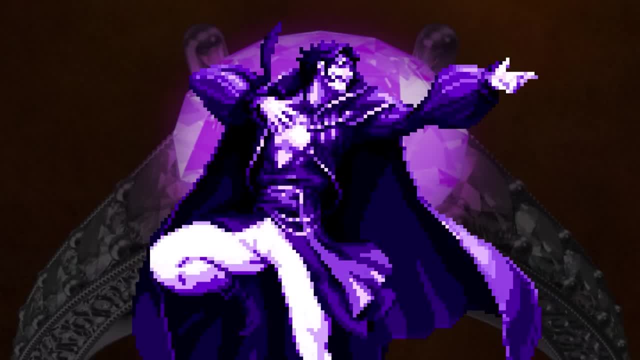 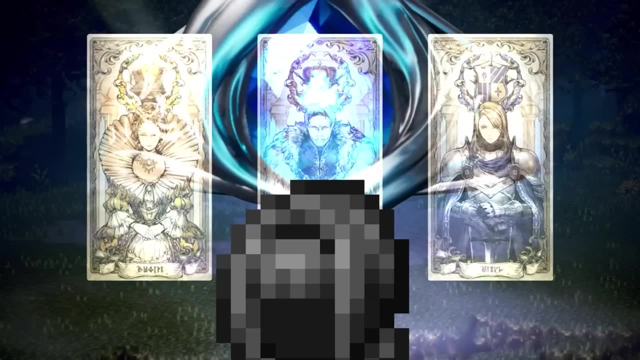 Auguste's ring corrupted him and forced him to follow not his own desires, but rather its own desires. The exact same choice that we find ourselves presented with at the start of the game: Pursuing one of three dark desires but never given the option to choose something else. 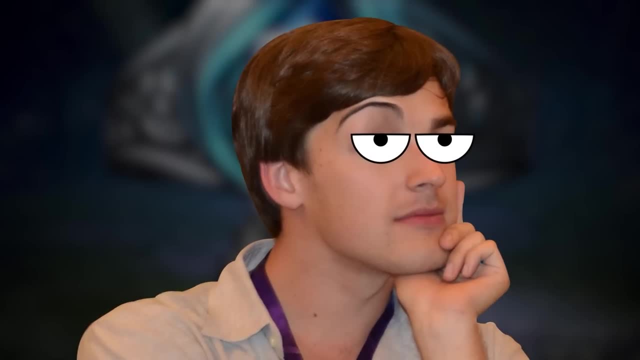 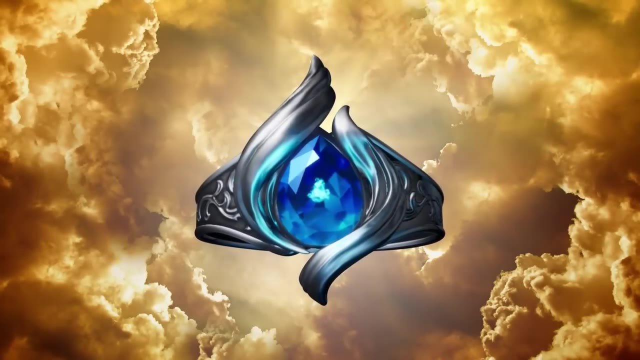 Okay, so clearly these rings have power over the user, but can I really say that they have their own desires? The answer is yes, Because these aren't just any rings. they're divine rings, Rings that came from a god or are god-like. Now, this is an important detail to keep in mind when looking at the final form for each of the game's major bosses. Each one is named after one of the eight primary gods from the original Octopath Traveler: Auguste becomes Prince of Thieves, Titus becomes the Thunderblade and Herminia becomes the Huntress. 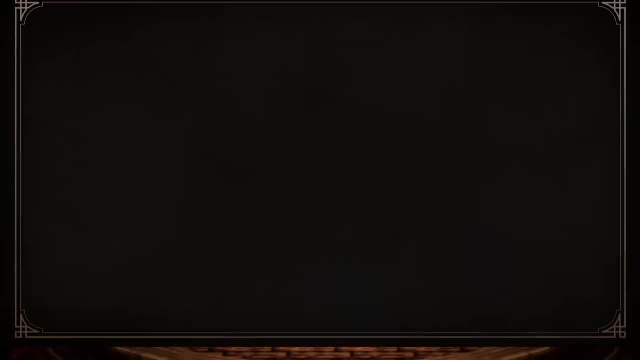 The exact same titles as three of Orstera's gods. We later learn that these rings aren't just powered by these specific gods. they are these specific gods, And it makes sense too. Brand the Thunderblade. Brand the Thunderblade. 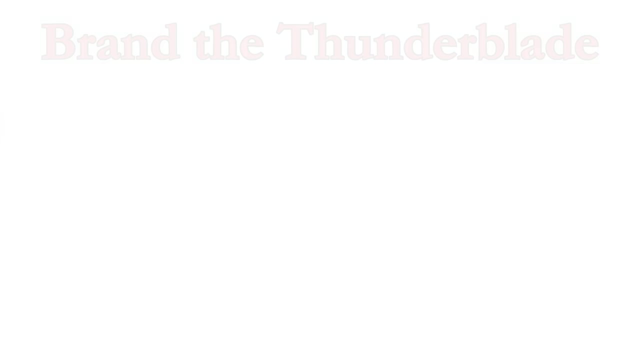 Brand the Thunderblade. The Thunderblade, for instance, is the god that offers the warrior class. in the original Octopath, Titus gets this ring and then pursues becoming an all-powerful warrior. So what about our ring then? 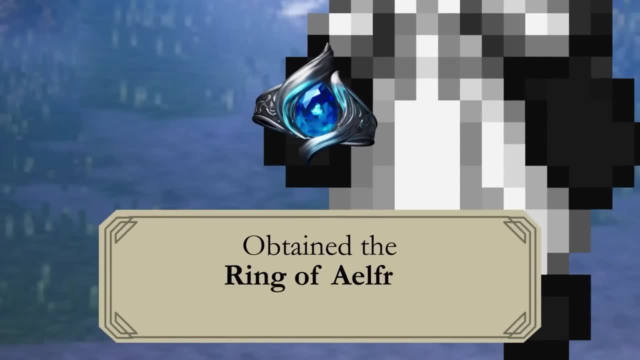 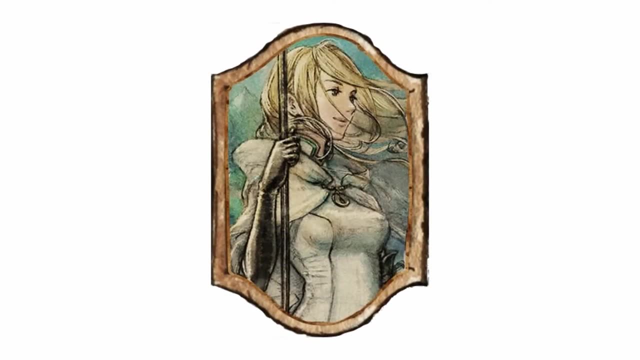 Well, after you beat the initial three villains, we're told that our ring is Elfric Flamebringer's ring. Elfric, like the other gods, grants a particular class in the original Octopath, the Cleric, Basically a white mage that specializes in healing and light magic. 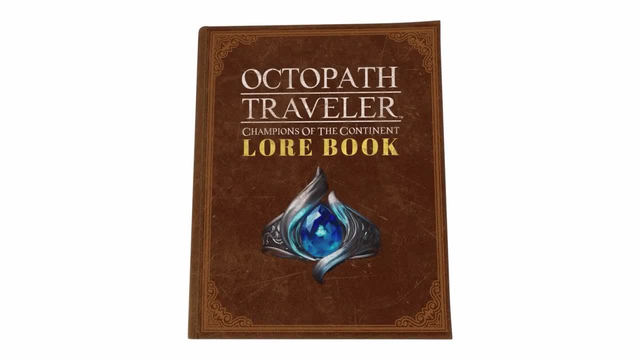 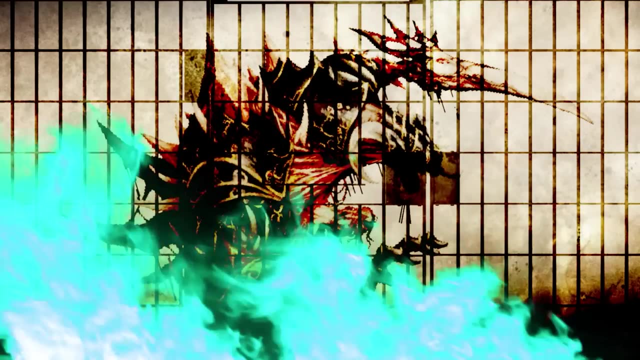 But Elfric is also one of the few gods where we get some of his extra backstory. You see, they're the one that imprisoned the evil 13th god by calling down fire from the heavens, which became known as the Sacred Flame. 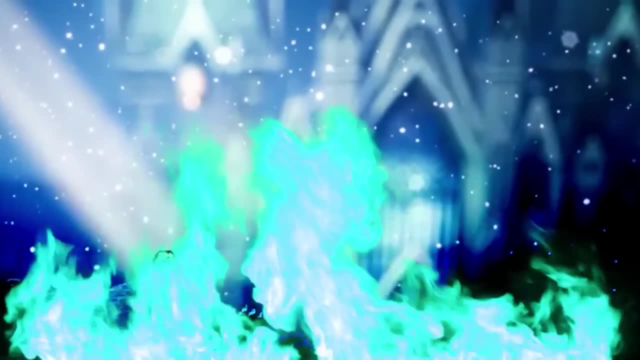 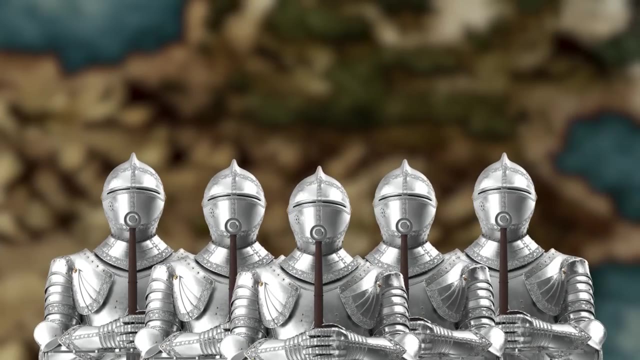 This led the Order of the Sacred Flame to be formed, an order which essentially runs the country. Although not all people are religious, the Order is super important to the running and governing of the continent. We see in the game that they have an army, that they can elect individuals into positions of power, like they do with Titus. 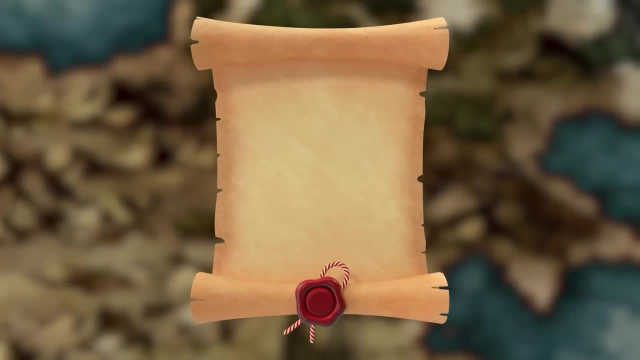 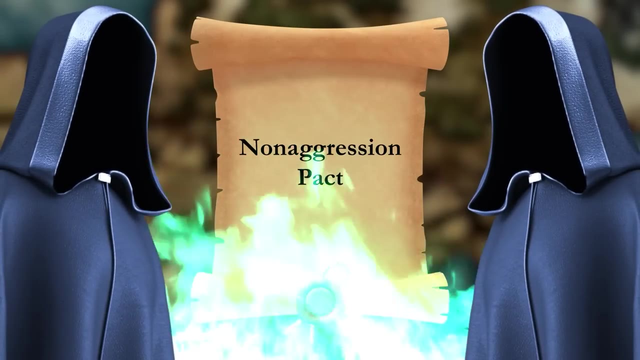 And in the Master of All Paths, we even discover that the Order supervised a non-aggression pact between the various kings of the continent. The Order runs this place. The priests of Elfric are the ones with all the power, But then suddenly, these other gods start using people. 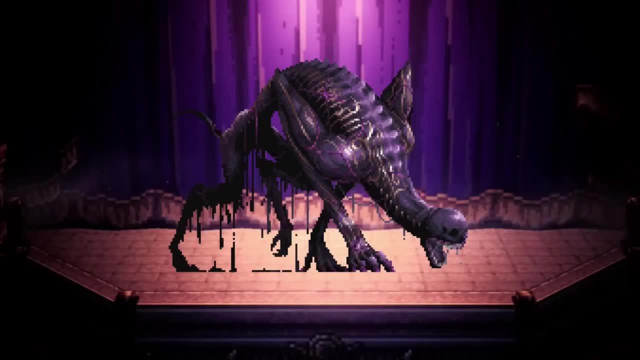 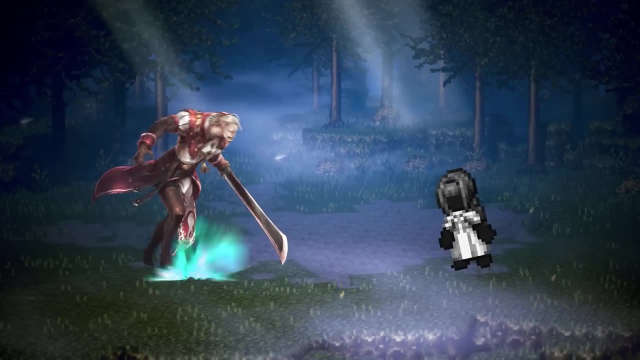 They start turning them into god-like beings in order to amass their own followings. Titus literally wants to overthrow the Order of the Sacred Flame. So what happens? Well, Elfric gets us to go in and re-establish the status quo. 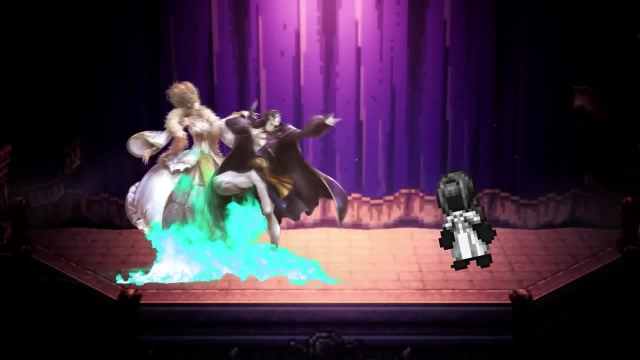 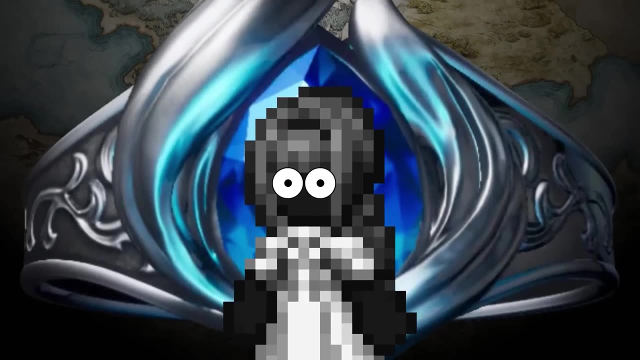 Stopping Titus' coup, pulling Auguste and Herminia from their positions of power to help restore the Order as the most important thing in the land. This isn't about saving the people. it's about making sure that Elfric is still the most worshipped god on the continent. 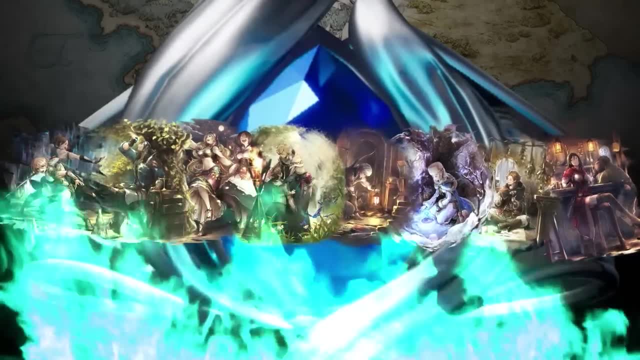 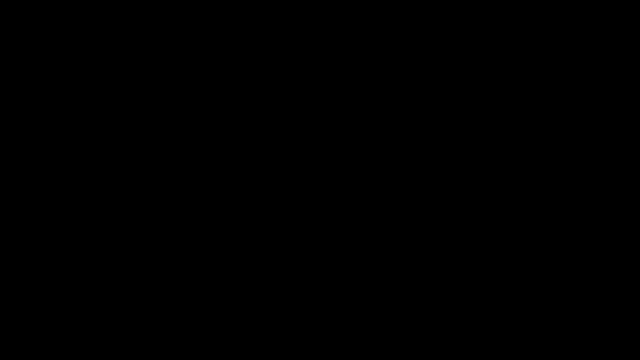 That's why it doesn't matter which character you start the game off, as You aren't the important one. As long as someone does the job, Elfric gets exactly what he wants. And if Elfric isn't all that great, maybe that 13th god wasn't so evil after all in the original Octopath. 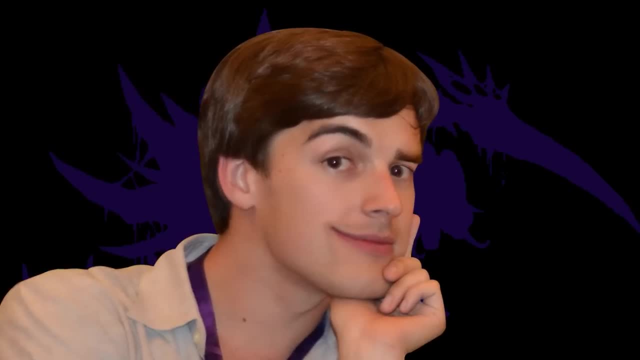 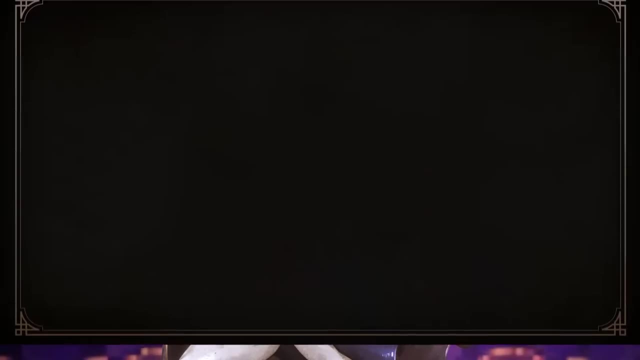 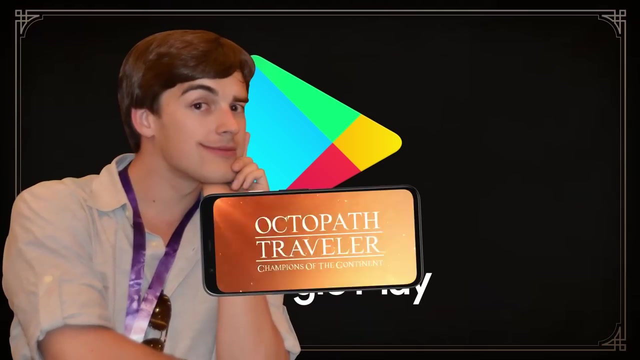 But that, my fellow travelers, is a theory for another day. In the meantime, remember, it's all just a theory, A GAME THEORY. Thanks for watching, And thanks one final time to Google Play for sponsoring this video. I love it when we get brand deals like this, because it gives me an excuse to make time for games that I wouldn't usually have a chance to talk about on the channels. 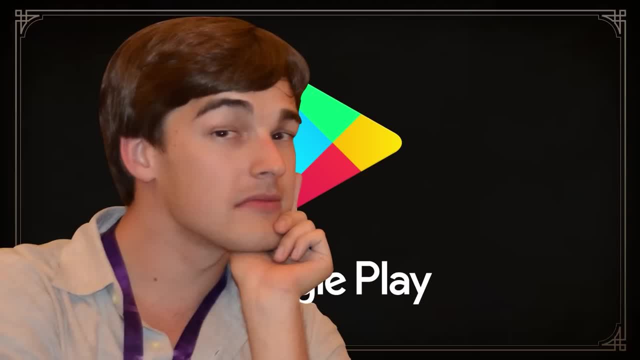 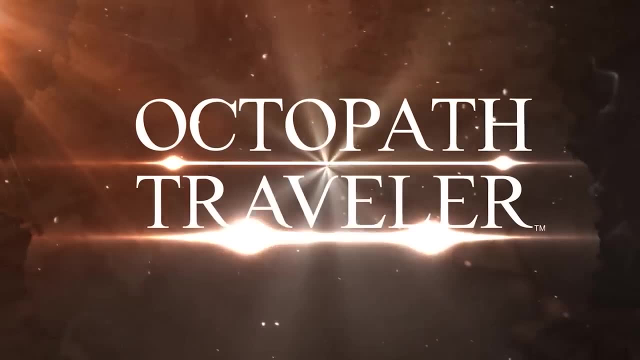 I grew up with JRPGs But haven't had much chance to play them lately because life is busy, you know. So when Google Play approached me and asked me to make a video about their latest releases, I jumped at the chance. Octopath Traveler- Champions of the Continent was a fantastic way to hop back into the genre.